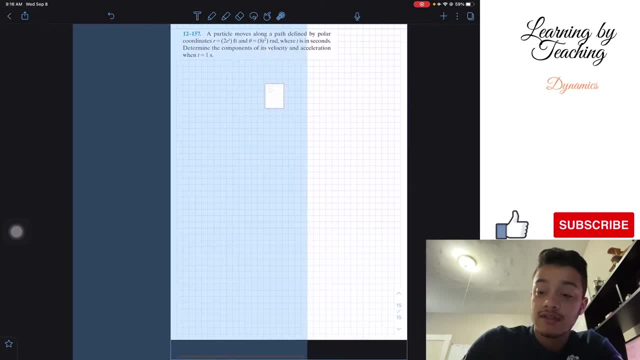 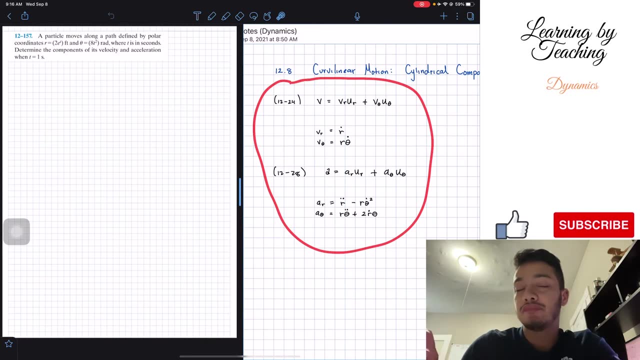 for this chapter. i created this little note in here because our velocity and our acceleration equations are a little bit, not complicated, not more complicated, but there have a little bit more, let's say, like components. so we have that our velocity has two components, which is the velocity in the radial component and in the angular component, and same thing. 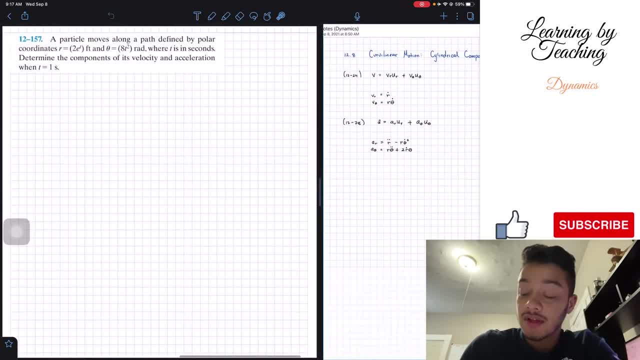 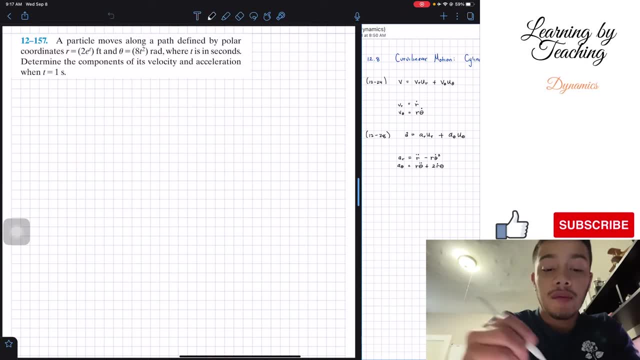 with the acceleration, okay, so i'm going to leave these notes in here, just so it could help us, and we're going to start the problem by first noting that. well, over here we have that the velocity should be either the derivative of the radial component or the theta component. so we're going. 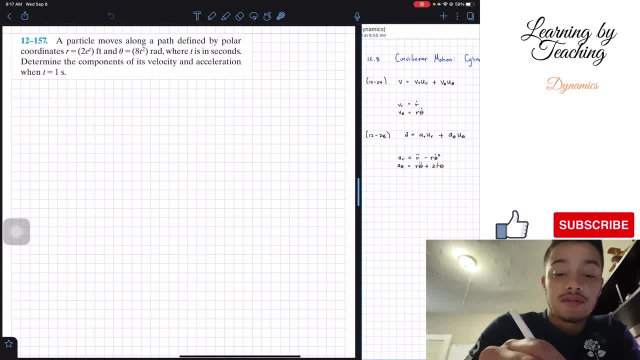 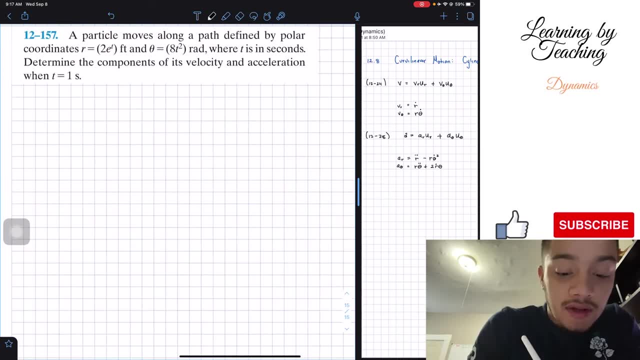 to do the first and the second derivative of the, our radius and our angle. okay, so let's start by doing that. we're going to have that r, this is equal to 2e raised to the t, and if we do, the second derivative of this r is going to be 2e to the t as well. okay, so not so so much of a. 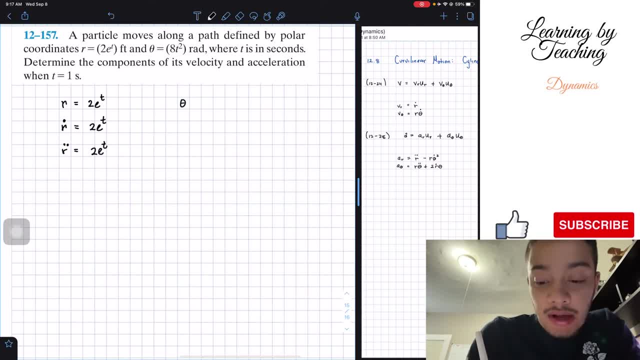 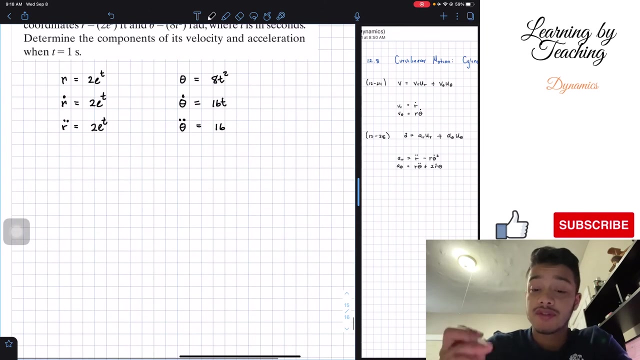 complication in this for this problem. and then we have also theta, which is equal to 8 t squared, and its first derivative is going to be equal to 16 t, and the second derivative will be equal to just a constant of 16. okay, so now that we have the first and the second derivative of these two equations, what we can do is we're. 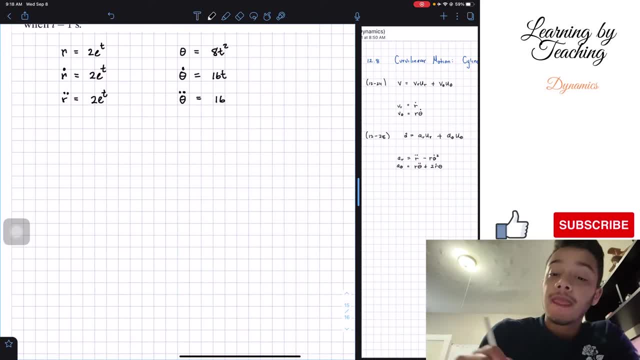 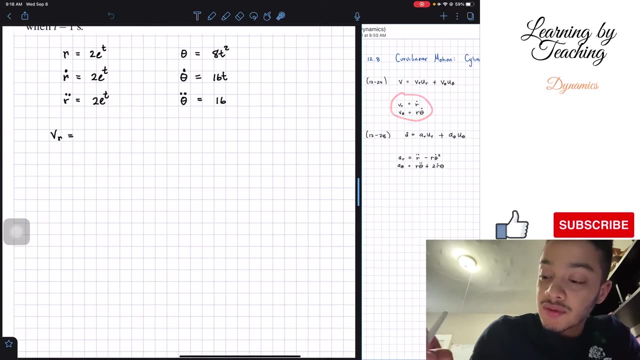 going to look at our equation sheet on our right in you and let's start finding our velocity and acceleration components. so let's start with the velocity in the radial component and, as we can see on the right in here, it's equal to the derivative of r. so the first derivative, which is equal to two, 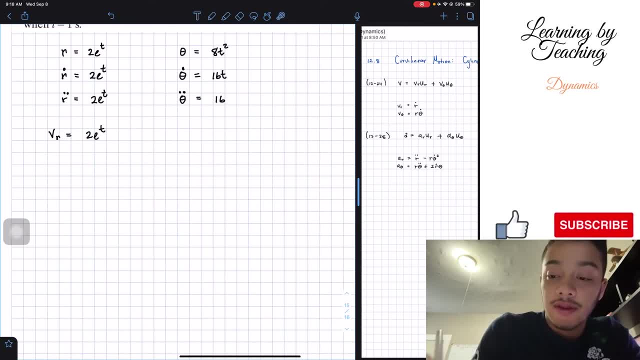 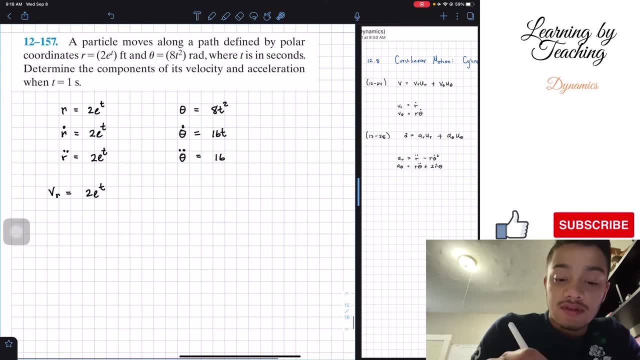 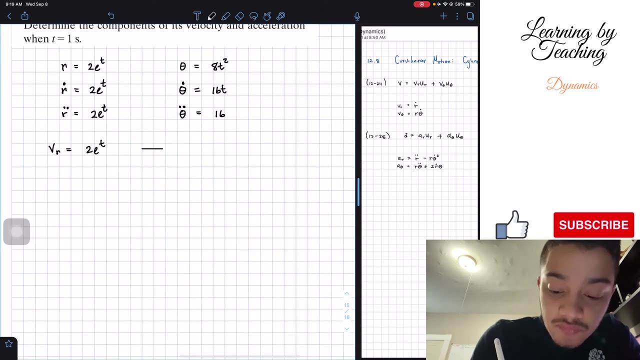 e to the t. as we can see in our above, we already made it okay. now the question is asking for this component when time is equal to one second. so what we're going to do is that we're going to say, okay, we are going to find this velocity when time is equal to one second, and this should be. 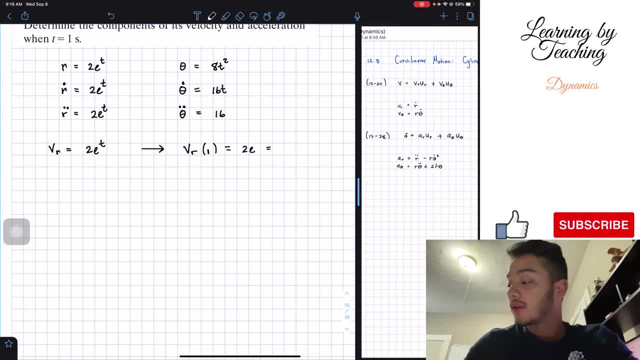 equal to just 2e. okay, and if we plug this into our calculator, 2e should be equal to 5.44. and then the units are feet per seconds. okay, i round out this number. next we can do the velocity in the angular component and we can realize that it's r times, so in here. all right, it's going to. 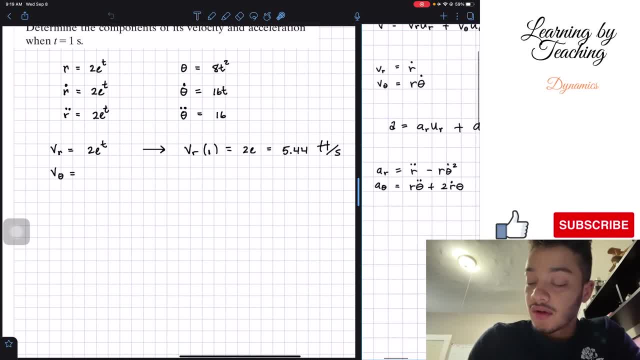 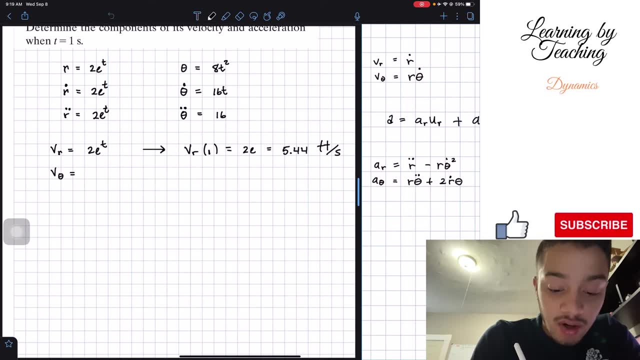 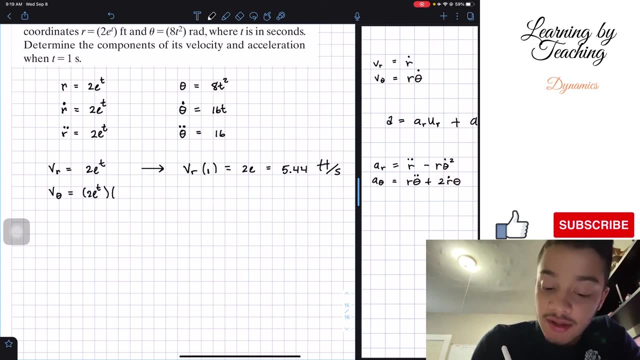 be r and- and i'm going to zoom in a little bit so it's clear- we have that. it's r multiplied by the first derivative of theta. so we have r, which is here, which is 2, e, t, and we're going to multiply it by the first. 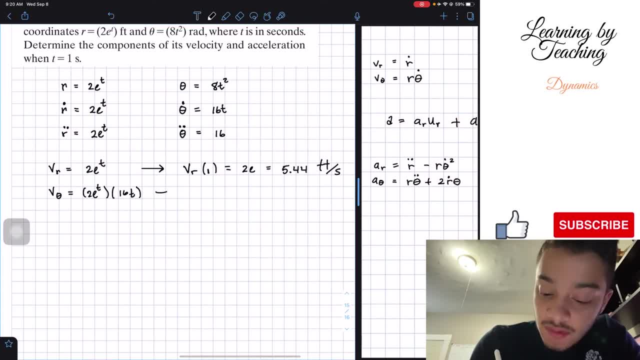 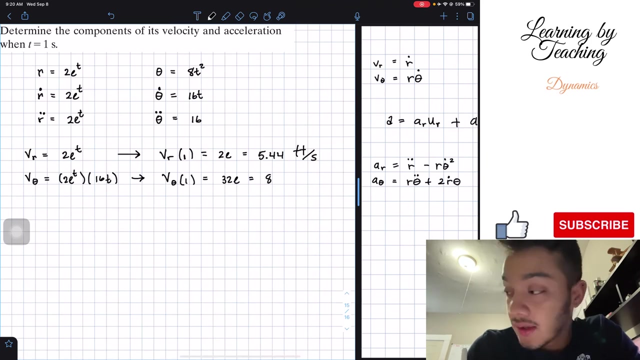 derivative of theta, which is 16 t. okay, now we're going to plug in when time is equal to one and we're going to have 32 e, and if we plug this into our calculator- so we got 32 e- it's equal to 86. well, if we round it up, it's going to be 87.0 feet per second. okay, and we're done with our. 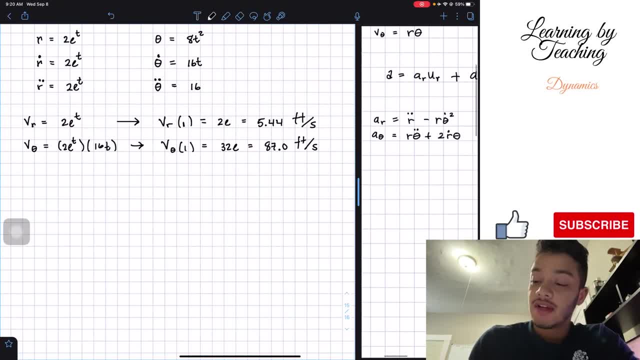 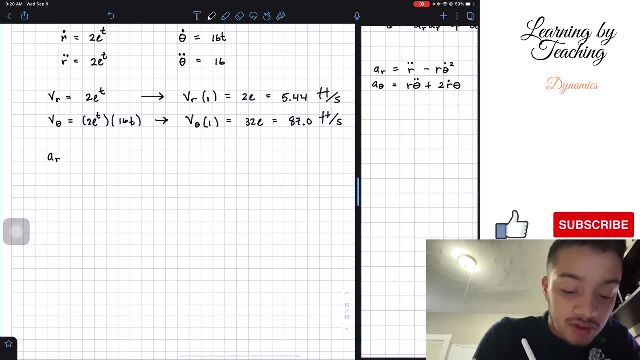 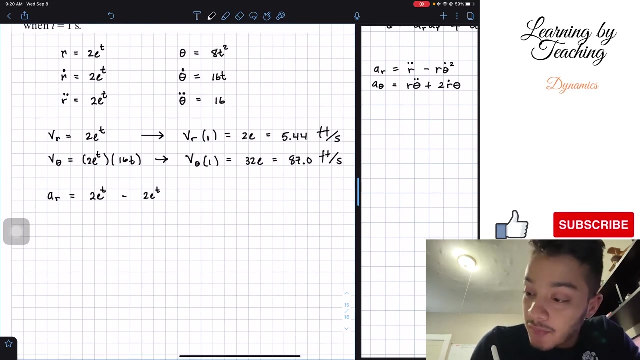 first answer for our velocity components. next, we're going to go and do the same thing for our acceleration components. so our acceleration in the radius component is going to be the second derivative of r. well, it's going to be 2 e t minus r, which is 2 e t in here, multiplied by. 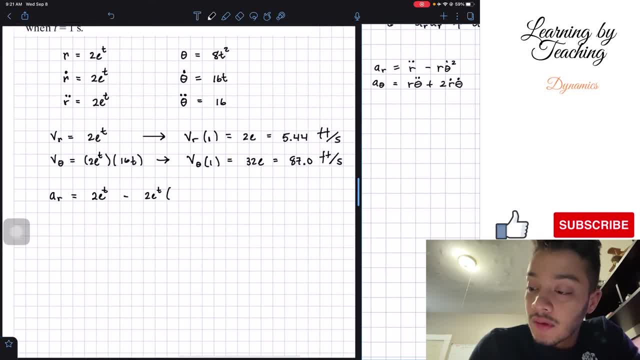 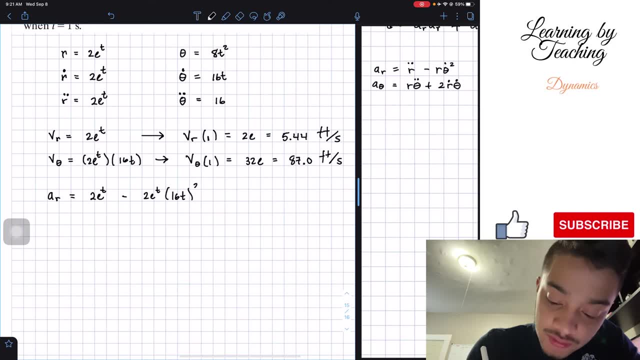 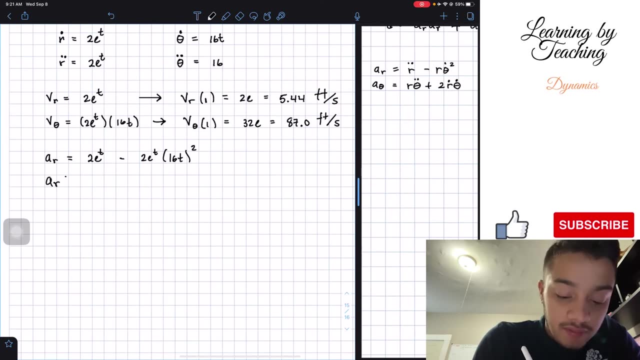 the first derivative of theta squared, which is 16 t, and we're going to square it like that, okay. so now what we can say is like: okay, if we plug in one as my term, we will have 2 e minus. we'll have 2 e multiplied by 16, a squared. okay. and if we solve for this, we'll realize well. 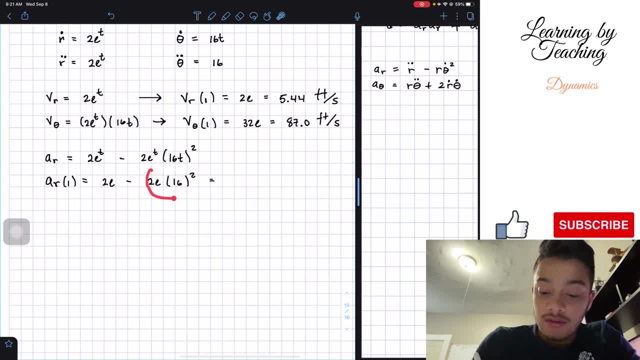 and here we got 2 e and in here this 2 e 16 squared. let's see how much is that. so we got 2 times 16 a squared, it's a total of 512. so these in here is equal to 512 e, and if we have 2 e minus this 512, we'll get negative 510 e. okay. 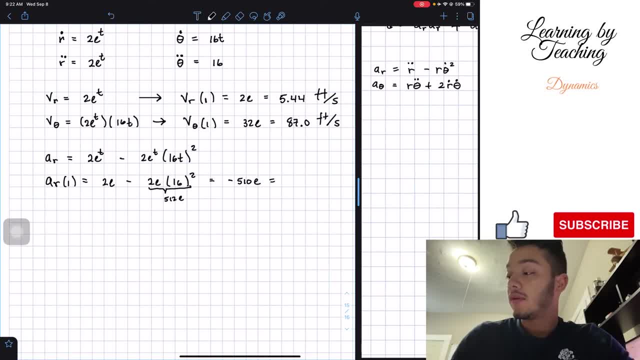 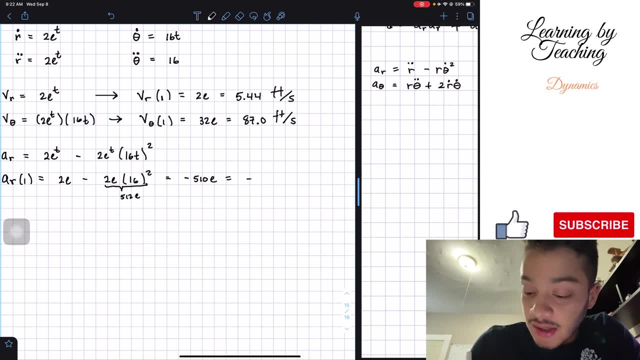 so we will put this into our calculator. we got 510 e, so we put this into our calculator. we get that this is equal to negative 1386 if we round. and this is a feet per second square because it's our acceleration. okay, it's our acceleration component, and then 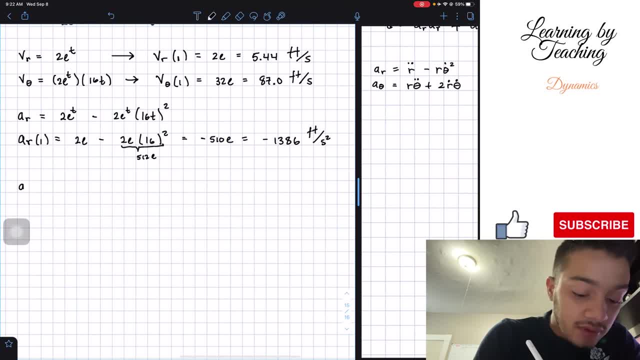 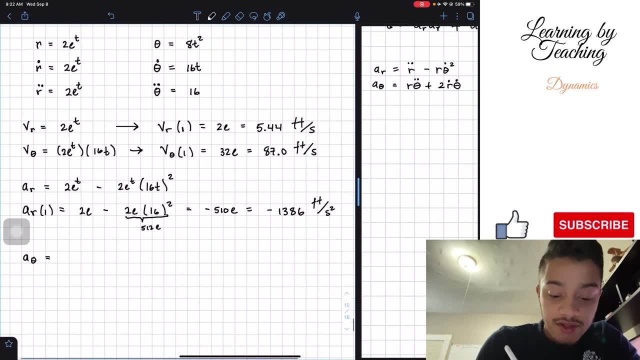 last we have, our acceleration in our angular component is going to be equal to r. well, r is equal to 2 e. so we got 2 e t and we're going to put this into our calculator. we get that this is equal to 2 e t multiplied by the second derivative of theta, which is equal to 16, and then we're going. 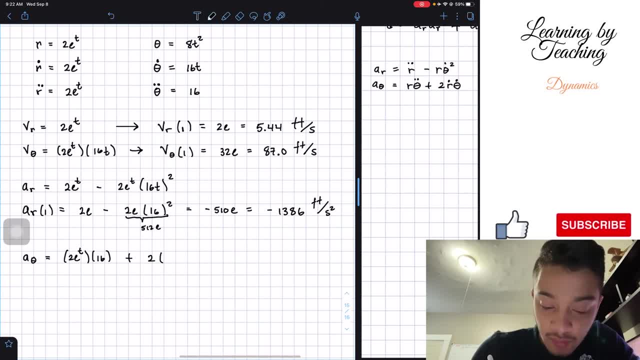 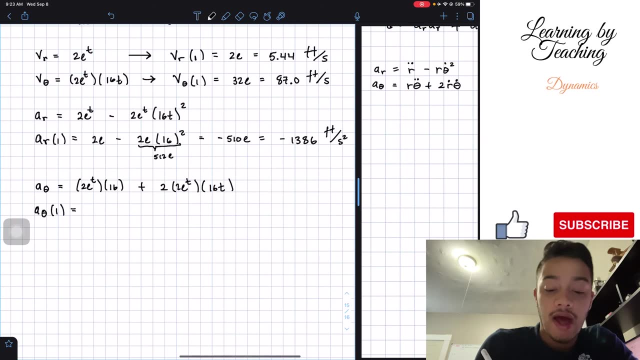 to add two times the first derivative of both, which is 2 e t, and then also 16 t. okay, now, if we plug in when our time is equal to one, what will we have? what we'll have in the first part? we'll have 32.. 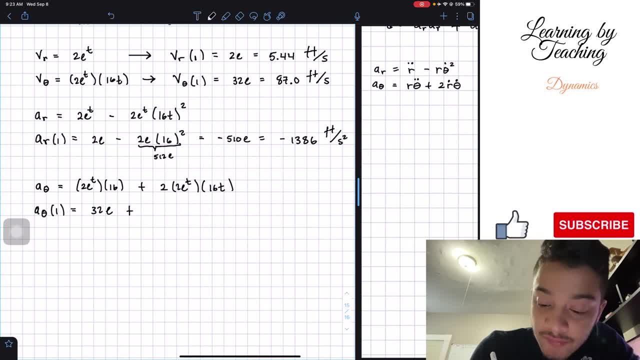 e plus, and then we will have 4 e times 16. okay, how much is 4 times 16.. is this equal to 64? so we can basically erase this and get 64 e. okay, and if we add them up- 64 plus 32- that should give me 96. 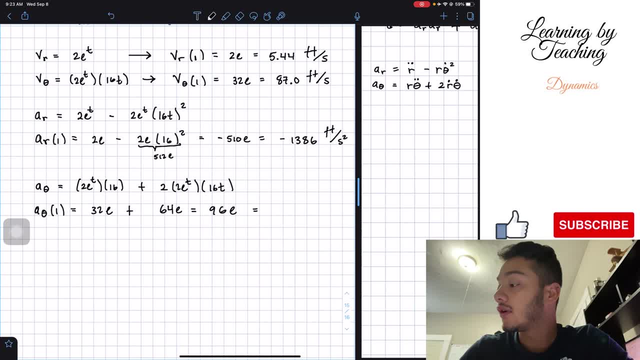 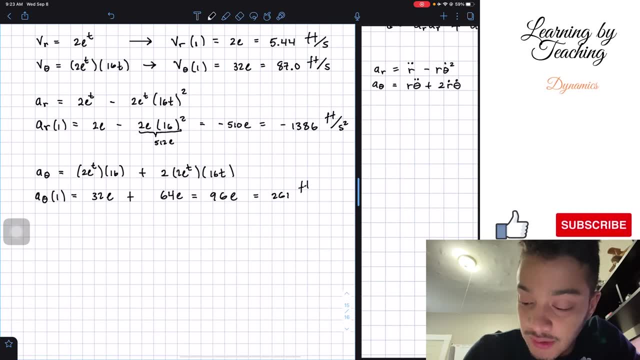 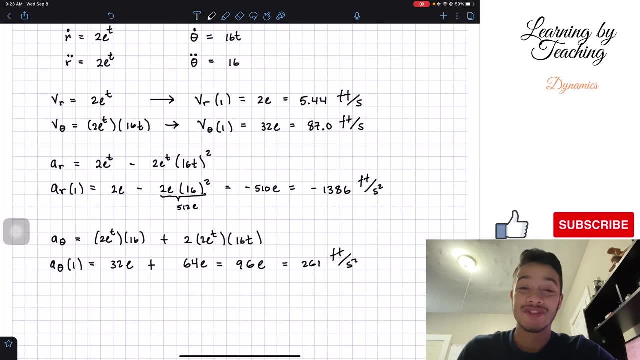 e and let's see how much this is into a calculator. in decimal point, this is equal to 261 feet per second square when we round it up. okay, so that was it for this video, guys. please push the like button, subscribe, and i'll see you guys in the next one. you, you.